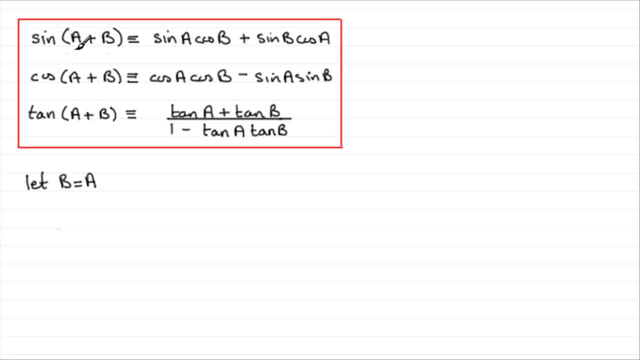 this identity. if we let b equal a, what we end up with is sine of a plus another a, because the b stands for an a, And a plus a is 2a, So we get sine of 2a, what is called a double. 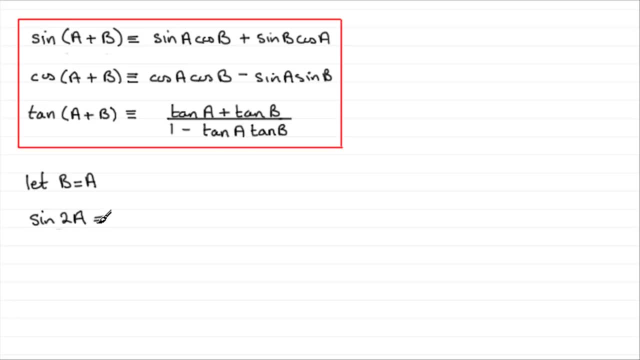 angle, And so that's going to be identical to sine a, and this b is replaced with an a. so we get sine a, cos a. Let's just write that in sine a, cos a, And then for this term b is it's replaced with an a. So we get sine a, cos a again. So plus sine a, cos a, Now we've. 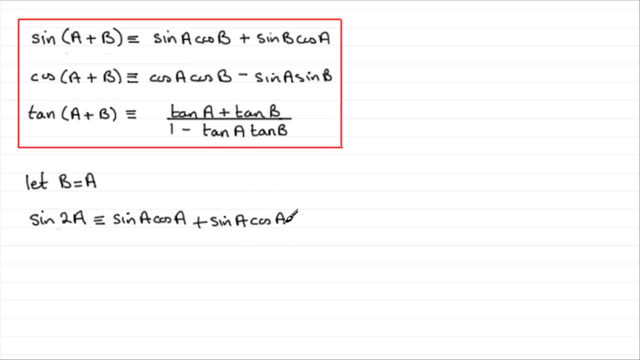 got two terms here exactly the same, So we end up with a result that therefore, sine 2a is identical to two lots of sine, a, cos, a, END, Arc, END, Numbers, END, Sy, inverse, P, ENDnew Sum, END crazy. think kim first identity that I would encourage you to learn Now if you forget these identities. 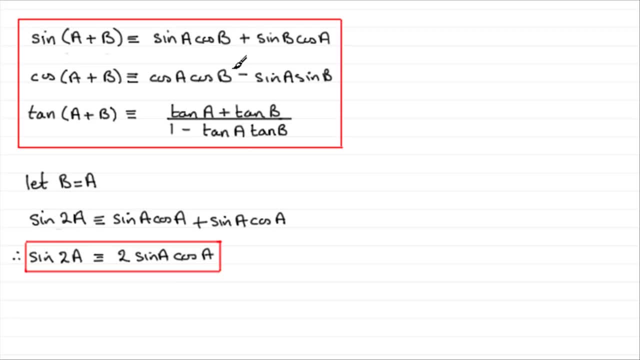 you can always build them up from these results. So it is your understanding that really matters here. Okay, well, I'm not going to do the cos one at the moment because that's a bit more involved, But you might like to try this one: The tan of a plus b, we know, is tan a plus. 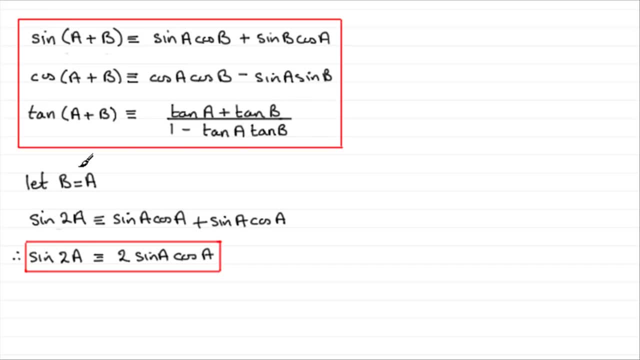 tan b: all over 1 minus tan a tan b. By doing a similar thing like this, you should be able to work out what the tan of 2a is, So maybe you might like to just give that a try. Okay, so let's see what we get. So if we replace the b with an a, we're going to have tan of. a plus a, which is tan of a plus a. So if we replace the b with an a, we're going to have tan of a plus a, which is tan of a plus a. So if we replace the b with an a, we're going to have 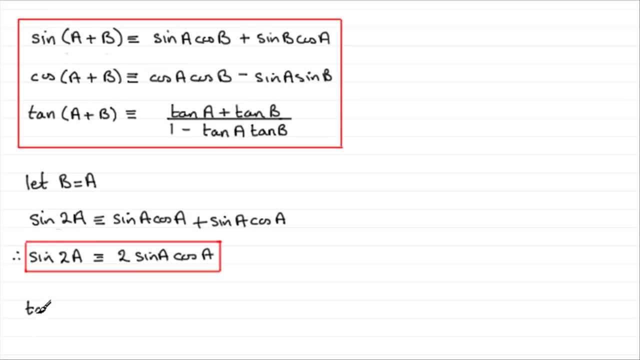 the tan of 2a. So tan of 2a is identical to tan a plus another tan a. So in other words, we have two lots of tan a on the top, And then all of this is divided by 1 minus tan a times another tan a, Tan squared a in other words. So on the 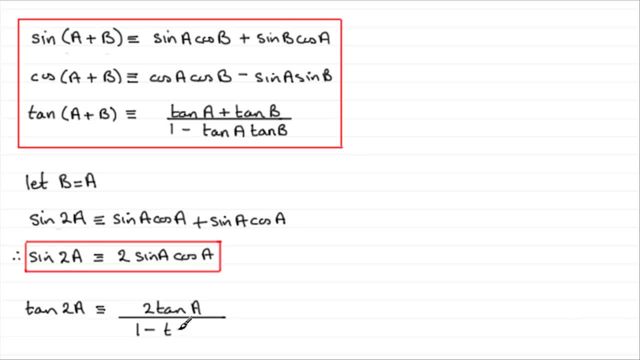 bottom. here we have 1 minus tan squared a, So it would be good if you got that one. Okay, let's just highlight this Now. I said I was going to leave the cosine one to the end because it's a bit more involved, So you might like to again have a go at coming up with an identity. 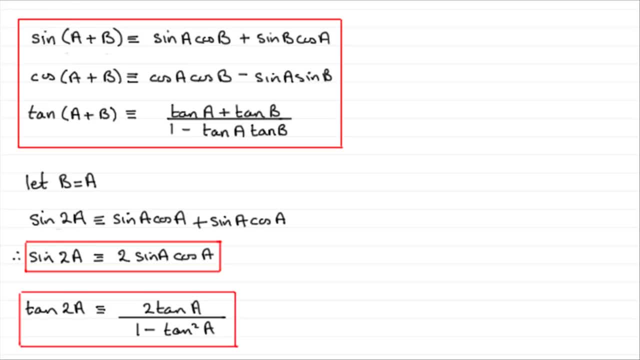 or two, And that's a little hint. Okay, so you might like to have a go at coming up with an identity or two. So you might like to have a go at coming up with an identity or two, And there are several identities that you can get for the cosine of 2a. Have a go See what you come up. 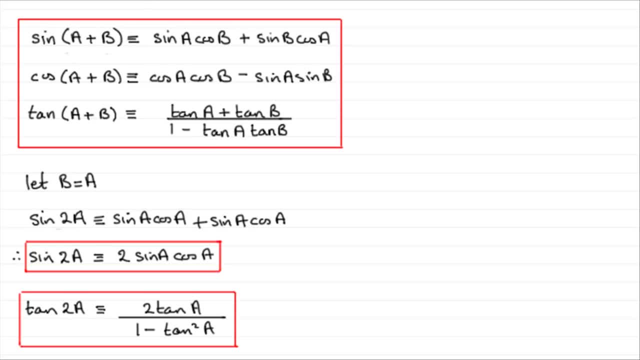 with: Okay, well, let's see, how did you get on. Well, let's start with cos 2a. then, where we replace the b with an, a Cos 2a is going to be identical. then to cos a times another, cos a, Cos squared. 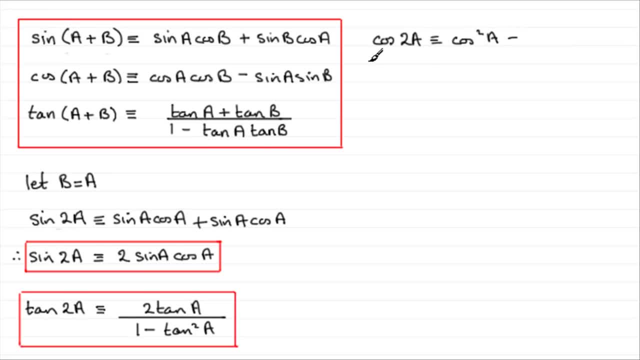 a times another. cos a Cos squared a times another. cos a Cos squared a times another. cos a Cos a, in other words Minus, and we've got sin a times another, sin, a sin squared a. So, did you get that identity? Well, if you did, well done. But what we can do is we can go on and 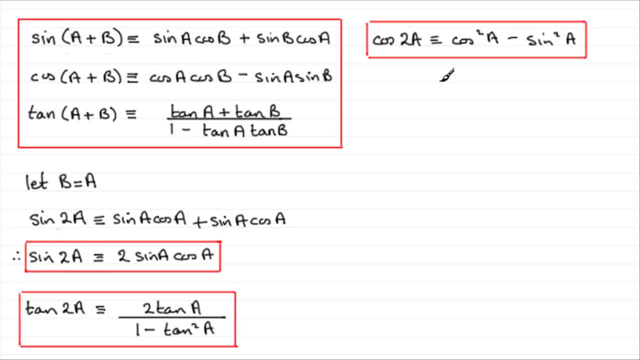 get more. And how can we do that? Well, we should know that sin squared of any angle, let's call it a plus cosine squared of any angle or cos squared plus sin squared of the same angle, doesn't matter which way around we have this always comes to one. We can use this. 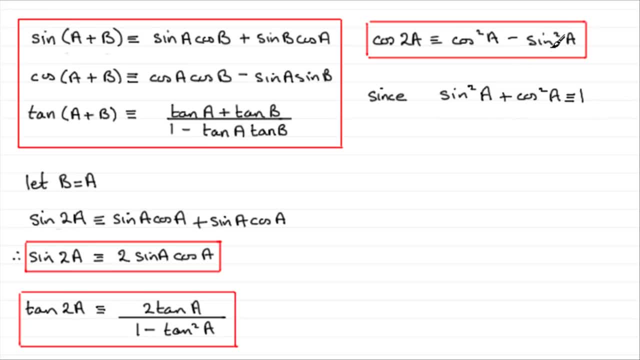 identity to change this result up here, Because, for instance, sin squared a, let's just write it in. if we were to rearrange this, sin squared a would be identical. And also if we made cos squared a, the subject would just say also, cos squared a would be. 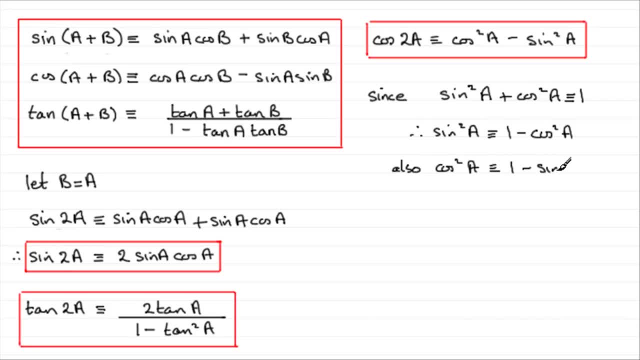 identical to one minus sin squared a. So what we can do is we could put this result into our identity up here. So what we end up with is if we replace the sin squared a a with 1 minus cos squared a in here. You've got to be very careful with this one Cos. 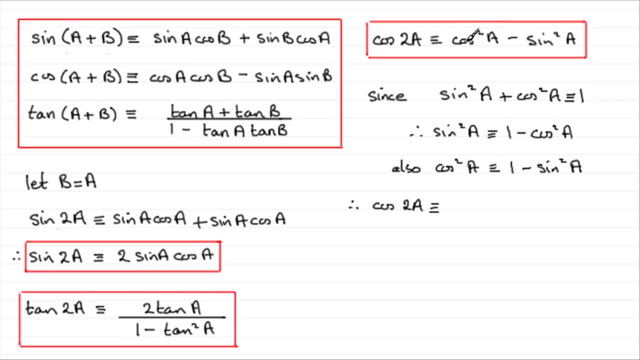 2a would be identical to the cos squared a here. and then we've got minus and then, replacing sine squared a with 1 minus cos squared a. There's a couple of terms here, so you've got to be careful. You've got to put that in a bracket. So if we open up this bracket, if 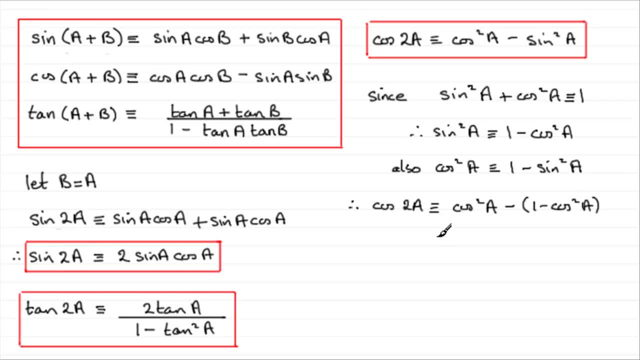 we expand it, multiply it out with the minus 1, that's here. what we end up with is that, therefore, cos 2a turns out to be cos squared a, and we've got minus, minus here, cos squared a, making another plus cos squared a. So we end up with cos squared a plus cos squared. 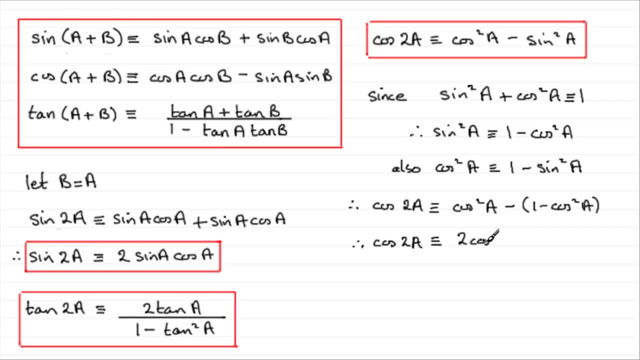 a, which is 2 cos squared a, and then we have this minus 1.. So we get this identity, this other version for cos 2a, An expression totally in terms of cosine. We can do a similar thing here again, only this time using cos squared a is 1 minus. 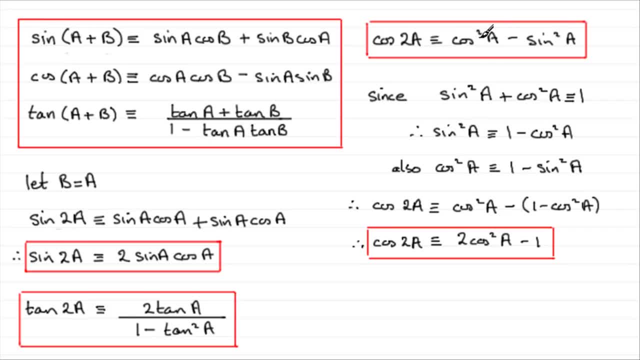 sine squared a. Put it into the formula here. So we also have that cos squared a is 1 minus sine squared a. Put it into the formula here. So we also have that sin squared a is 1 minus sine squared a. Put that into the formula here. So let's. 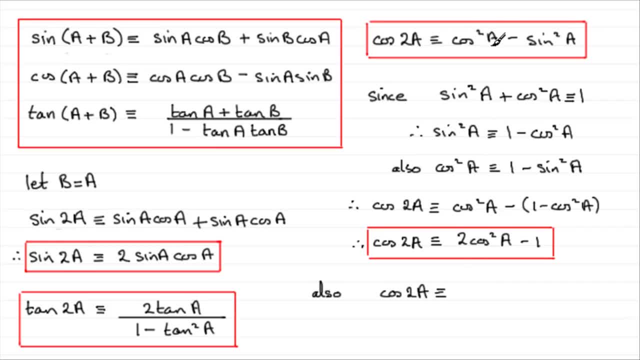 get rid of the remaining 2. cos squared a were nothing, and we also have 1 minus a. Never erase this whole formula if you don't remember not to delete it. So therefore, cos squared a would be identical to. so, in place of cos squared a, we've got.